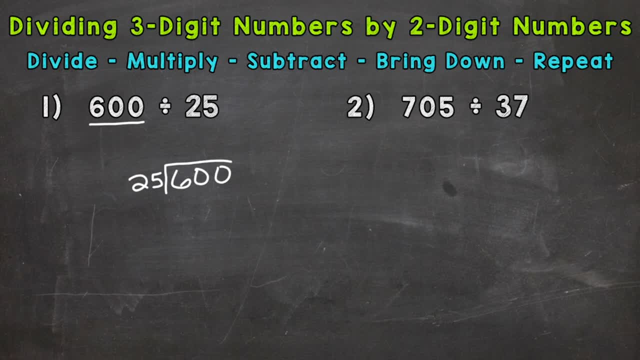 So let's start our process: Divide. So we need to do 6 divided by 25.. Well, we can't pull a whole group of 25 out of 6.. I'll underline the 6 I'm talking about. That's 6 there. 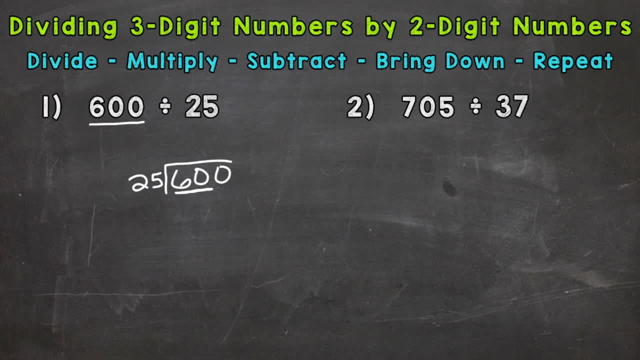 So we need to look at 60. We can use two digits there, So 60 divided by 25.. How many whole groups of 25 can we pull out of 60?? Well we know, 2 times 25 is 50.. 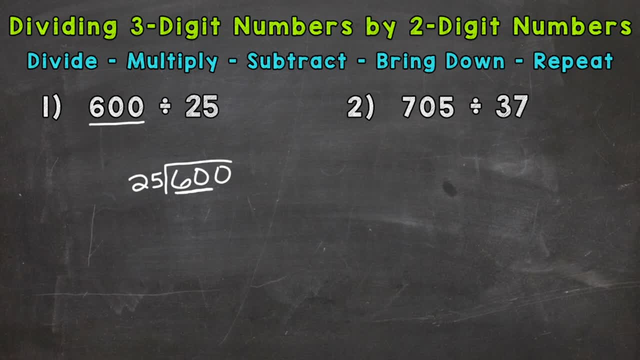 Okay, so pretty close there. And if we were to do 3 times 25, that's 75. So that's too much there. So we can pull two whole groups of 25.. So that was our divide step. Now multiply 2 times 25 is. 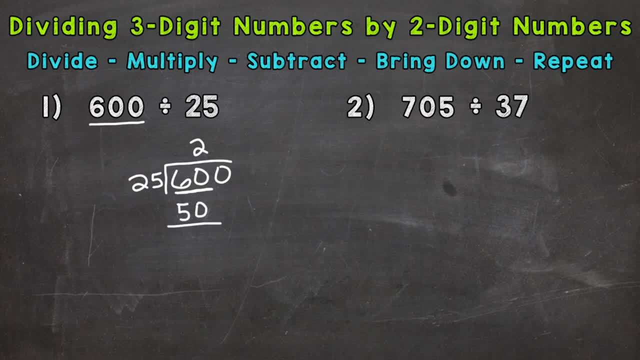 50. Then we subtract and we get 10.. Bring down our next digit, which is at 0, and we have a hundred there. So now we repeat those steps. So divide 100 divided by 25.. So we can think: well, 25 times 4 hits a hundred. exactly. So we can pull. 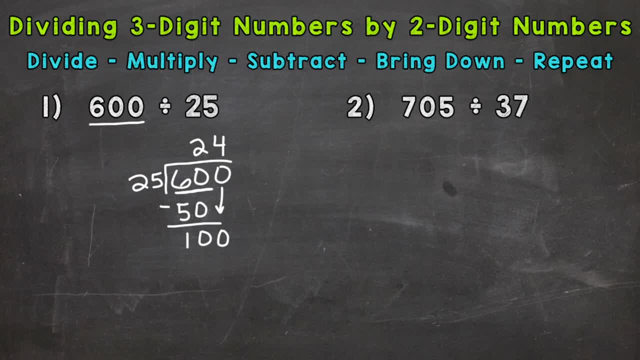 four whole groups of 25 out of 100. Now we multiply, We get 100. here Subtract We get 0. And that brings us to bring down. But we went all the way over to the ones place and there's nothing else to bring down. 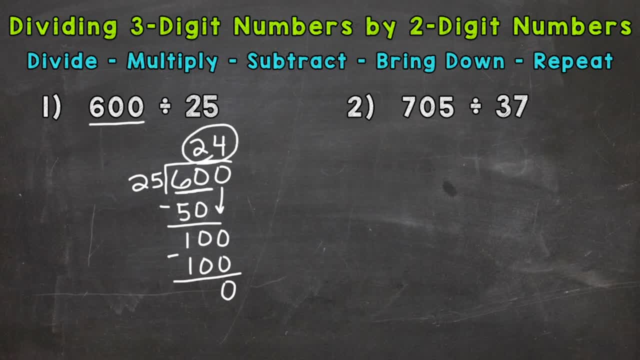 So we are done: 24 is our answer and we do not have a remainder. So on to number 2, where we have 705 divided by 37.. So let's set this up first: 705 is our dividend and 37 is our. 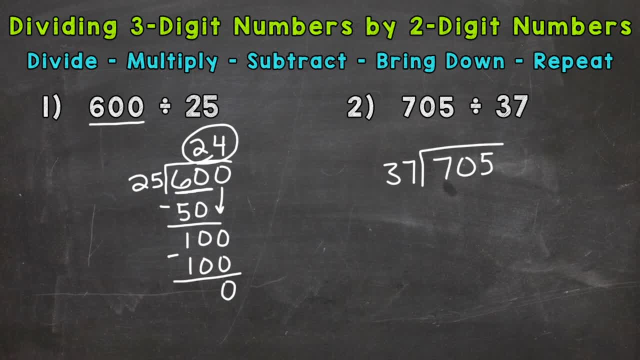 divisor. Now, if you forget the words dividend and divisor, that's okay, but knowing that 705, that first number needs to go under the division bar and the second goes outside- is the most important part. So let's go through our. 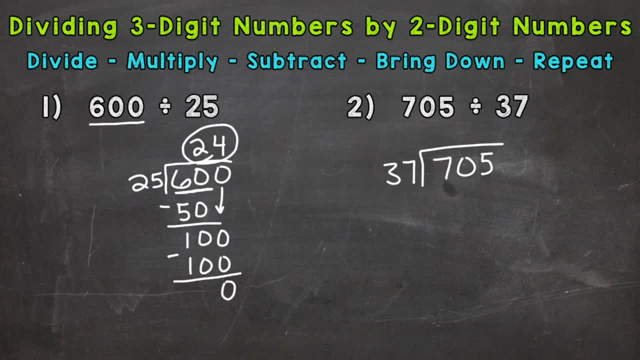 steps: Divide Well, 7 divided by 37. Can I pull any whole groups of 37 out of 7? No, So I need to look at 70. So how many whole groups of 37 out of 70? 37 is. 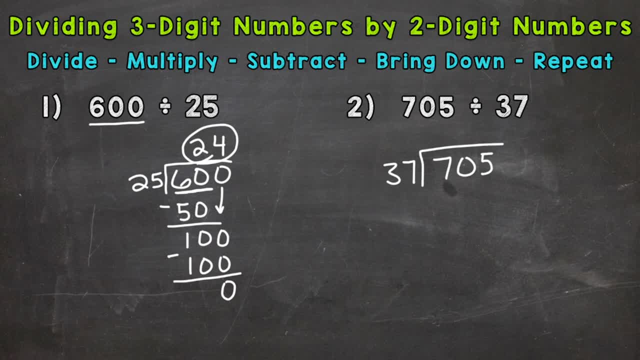 not a very friendly number to work with. so we need to estimate and check because we probably don't know the 37 multiplication facts off the top of our head. So a couple of strategies we'll go through as we work through this problem. 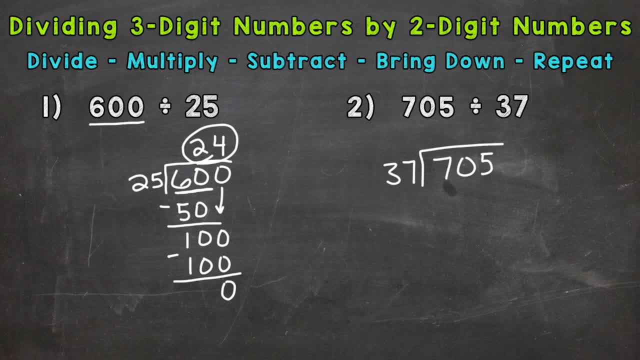 So I would suggest rounding to a number that's easier to work with to get an idea of where to start. So I could think: well, 37 is close to 40, so let's round to 40,, the nearest 10.. 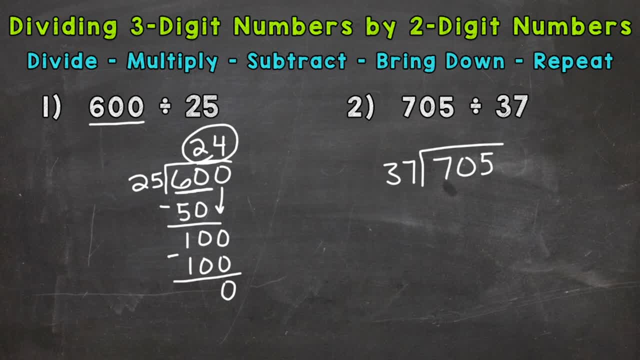 Well I know 40 times 2 is 80. That's kind of close to 70. Why don't we try 37 times 2 to get us started here and see how close we get? 37 times 2 gives us 74. Pretty close, but. 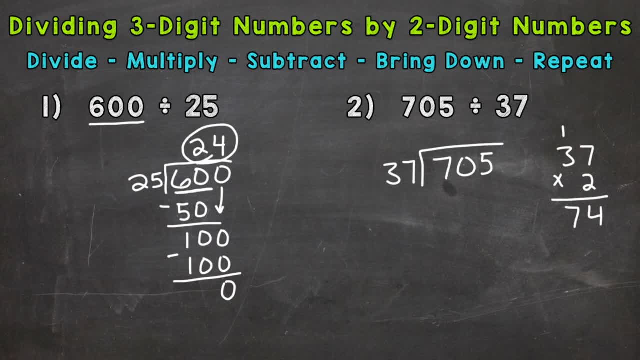 we went over. so we can't pull two whole groups of 37 out of 70. We can only pull one. 1 times 37 is 37. Now we subtract Need to borrow in this one: 10 minus 7 is 3.. 6 minus 3 is 3.. So we get. 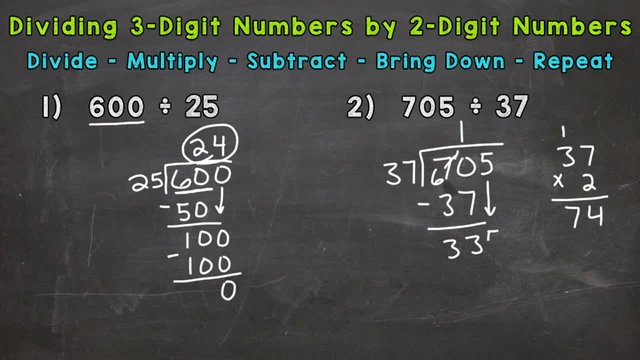 33.. Now we need to bring down our 5, and we end up with 335, and let's repeat our steps. So we go back to divide. Hmm, 335 divided by 37. How many whole 37's out of? 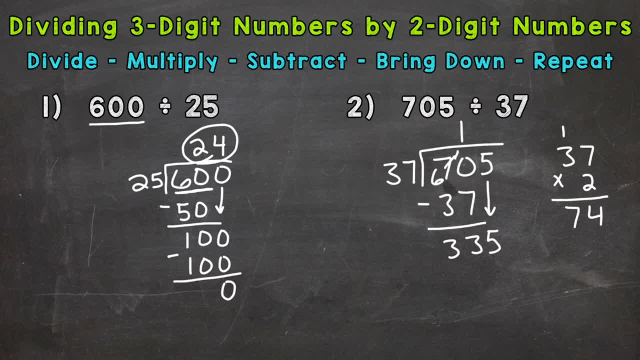 335?? Well, another strategy, we can use something we know and in order to gauge what we can try. so we know, 37 times 10 is 370.. that's kind of close to 335, so we can start with something around 10.. let's try eight. so 37 times eight, just to see how close. 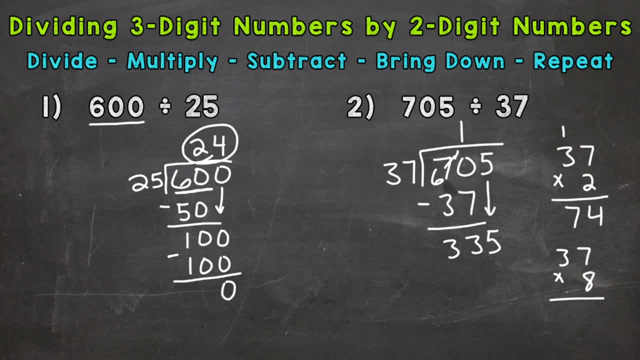 we get. it doesn't hurt to try something out. you can always try something else if you didn't get close enough, are you? or if you went too far over. so 8 times 7, 56, 8 times 3, 24 plus 5 is 29 296.